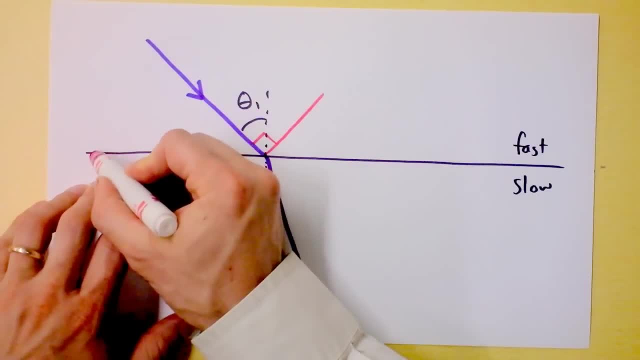 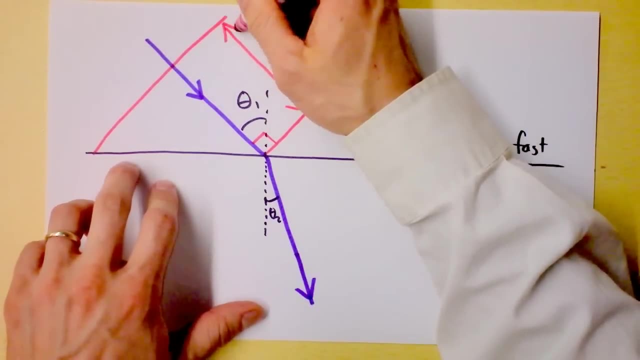 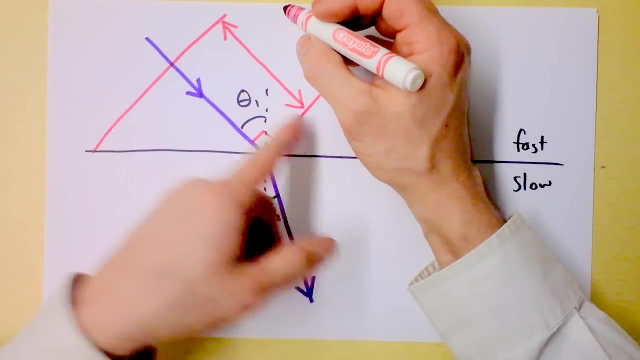 corresponds to it. and here's another one, here's another wave front and I want to say that this distance between these two particular wave fronts, it could be a wavelength, it could be many wavelengths, I don't really care. I'm just going to say that the distance the wave goes in that time is the velocity of the wave. so 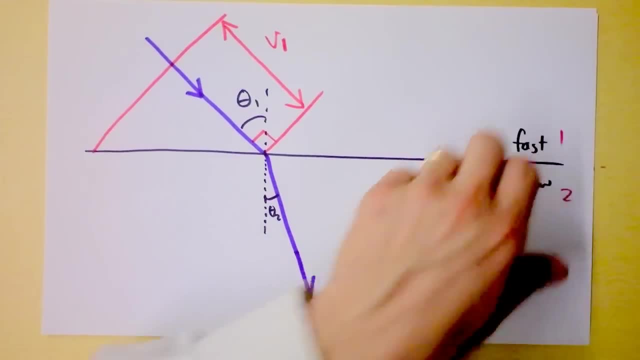 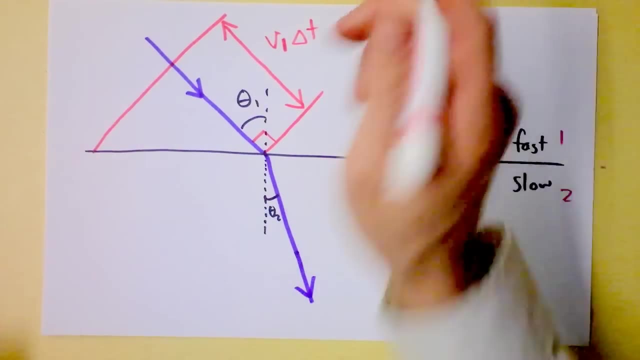 I'm going to call it v1 here, so one is up there and two is down there- v1 times the amount of time that it's taken to go that far. but the frustrating thing is that the guys in this slow region- you can think of it as a swamp or whatever you want to do- have not. 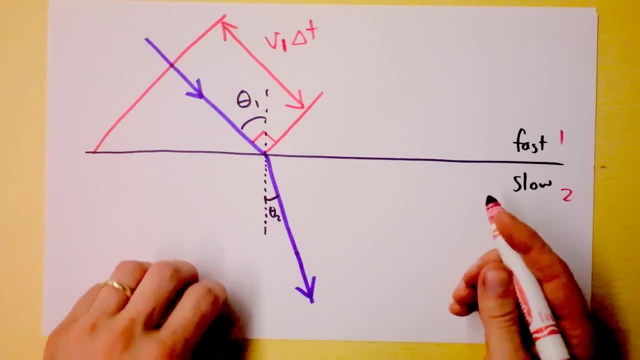 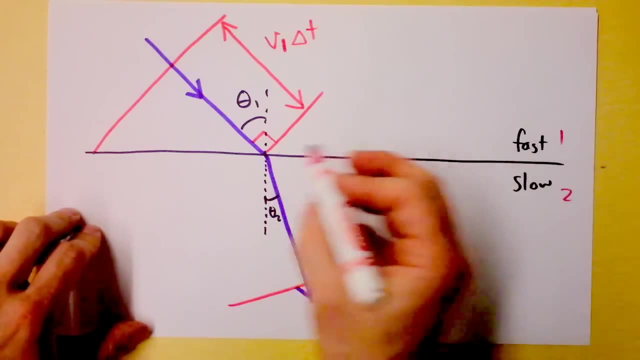 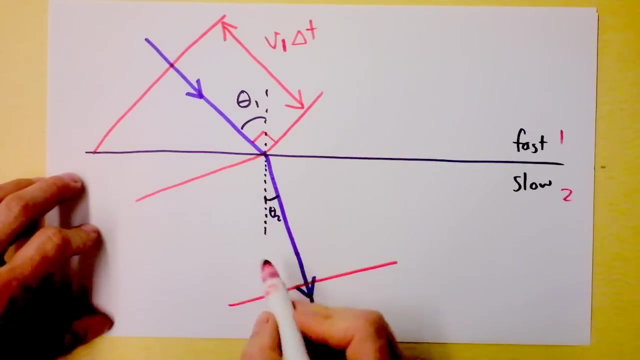 been able to go nearly as far. And so we say that Their normal looks something like this: Because they bent this direction and I'm interested in how far they went during the same amount of time. it looks like they only went This far. you see that this line has to be parallel to that line, it has to be normal. 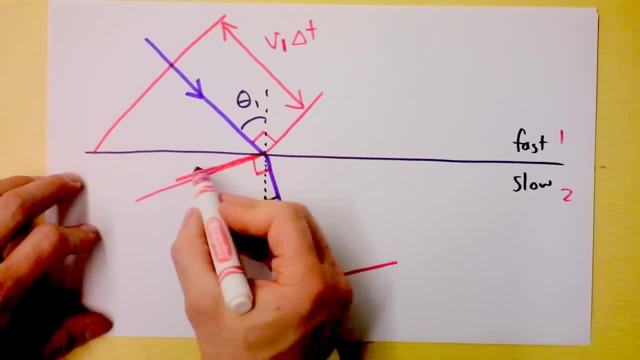 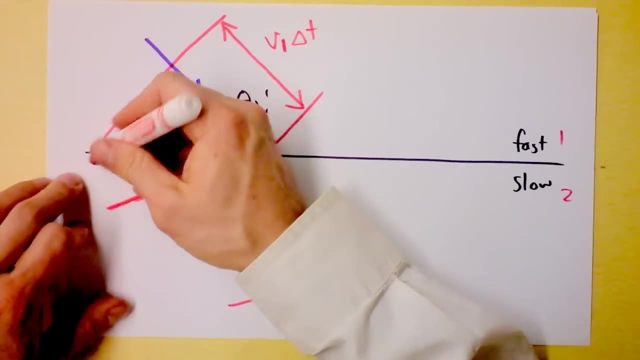 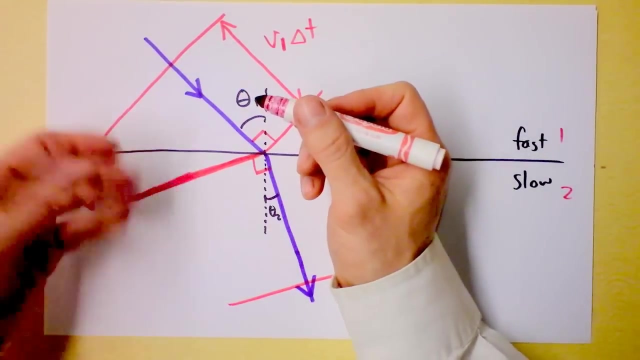 to that line right there. I'm going to come out here like this, maybe, And investigate how far they've gone. as soon as I get to a normal, I can say that this is the time, this is the distance that these guys at this part of the 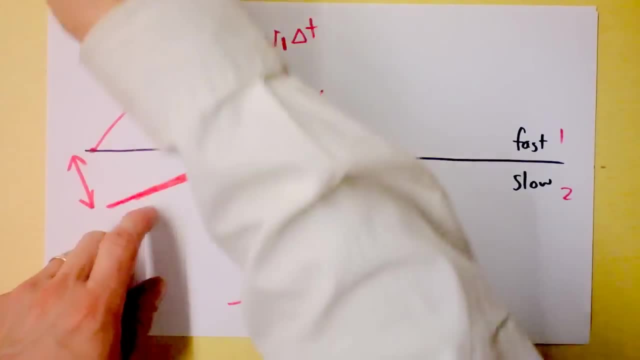 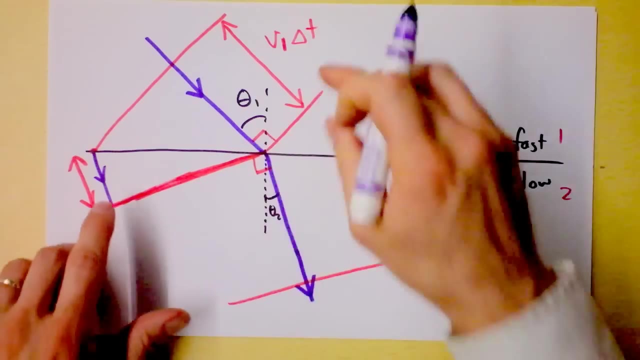 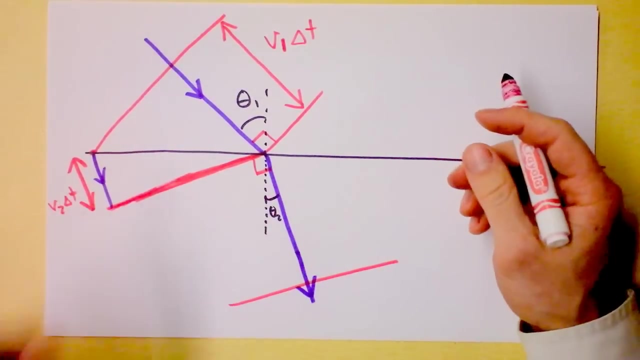 wave have gone. this is a little bit weird, but I guess I'm going to have to draw myself a little line. Oh right, this is the normal. so that's how far those guys have gone during the same amount of time. Now, this must be. therefore, this must be v2 times delta t. do you see how this triangle? 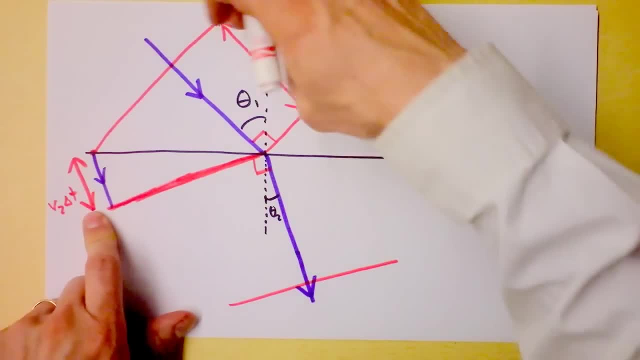 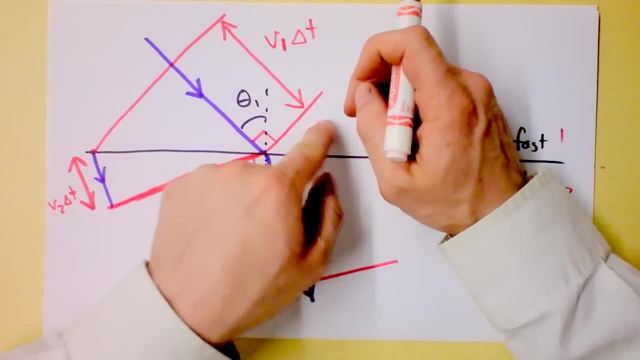 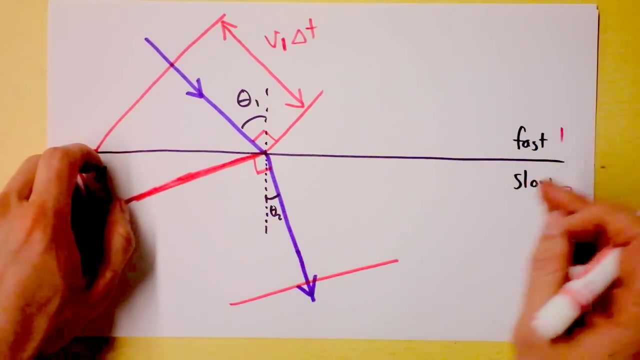 is, has A A leg at v2 delta t and this triangle has a leg at v1 delta t during the same amount of time, whereas this guy would have gone this far had he been out in the fast region because he's in the slow region. he's only gone that far because he's in a swampy slow region. 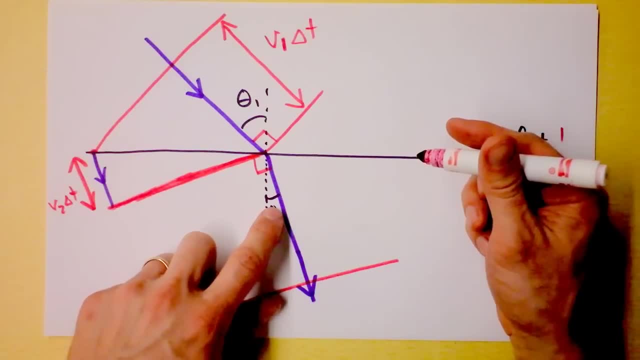 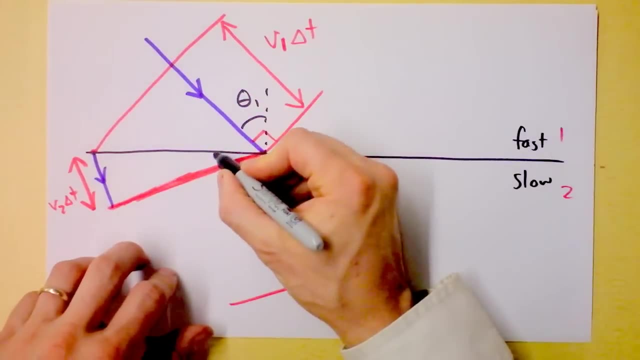 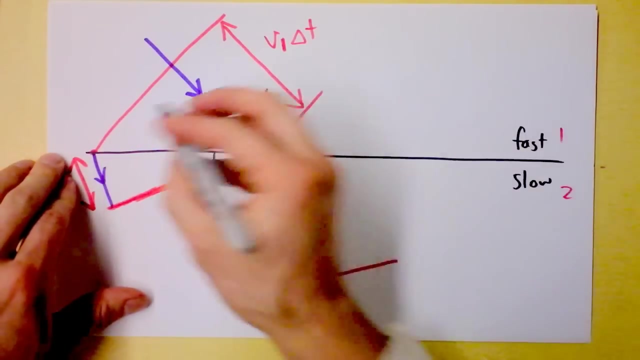 Now it's time to make ourselves a little bit of angles. this is pretty fun. This is theta two right here, but the magical thing about it is that this is also theta two right there. You prove that to yourself. check it out. This is also theta two, and while this is theta one, turns out that this also has to be theta. 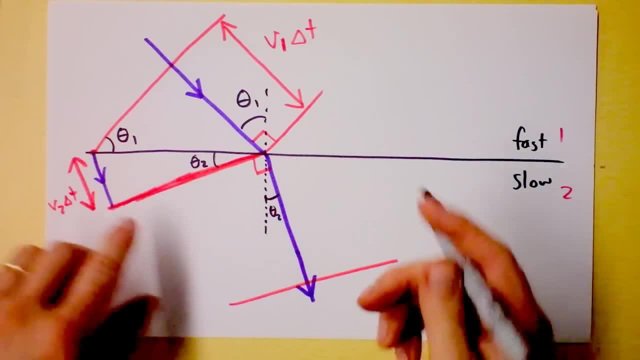 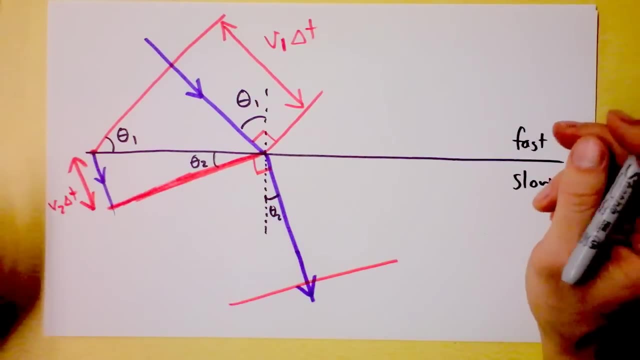 one. Oh interesting, you saying something about triangles. you saying like: this is theta two, this is the complement of theta two. we can make a dotted line down here and make all kinds of things. Oh my goodness, geometry is so beautiful. But here's my point: if this is a right angle- and this is a right angle, of course it is. 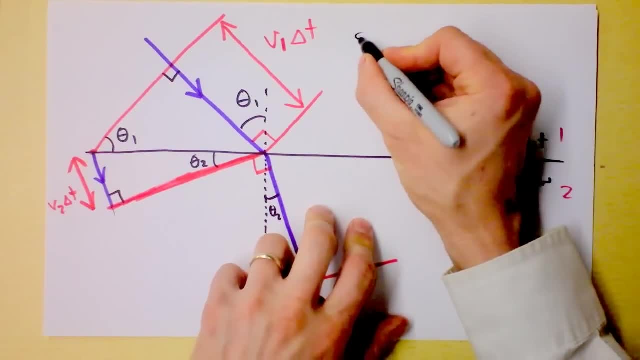 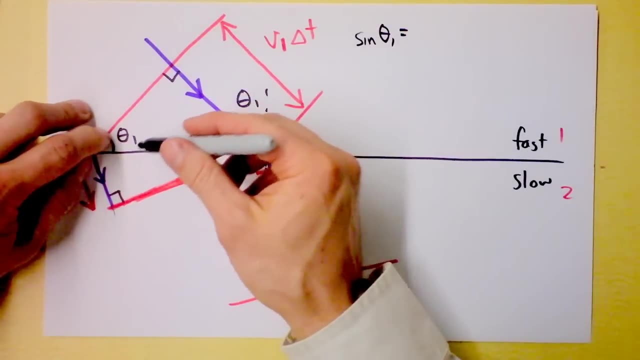 because those are right angles also, then I can make the statement that the sine of theta one, well, sine of theta one, here's theta one, and it's in a triangle, so I'm going to say that it's the opposite over the hypotenuse. well, that's this sucker right here, vi times. 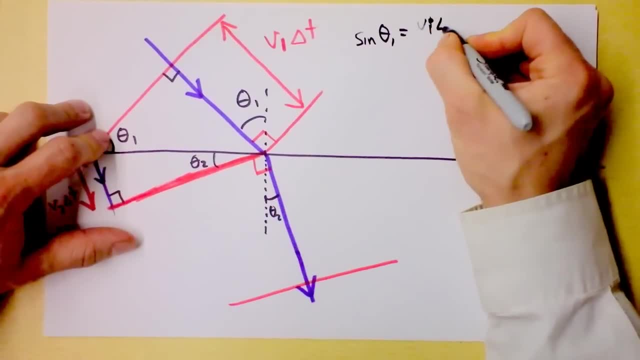 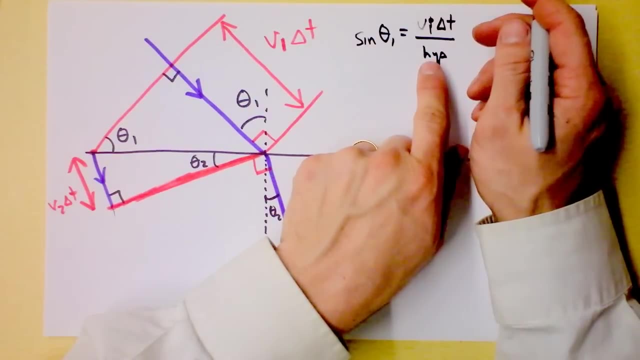 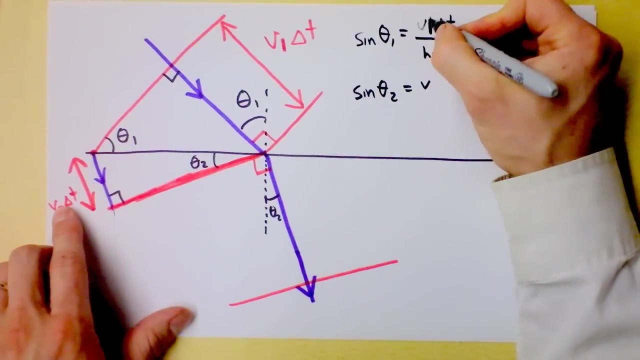 delta t, vi times delta t divided by the hypotenuse. well, the sine of theta one: oh, shoot, okay. and this is the sine of theta two. It's going to be v. no, I didn't mean to say vi, I mean to say v one. 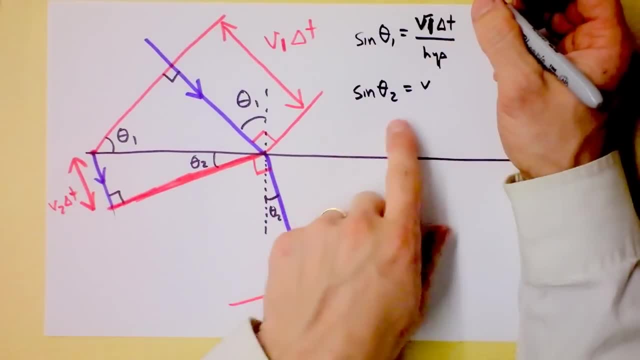 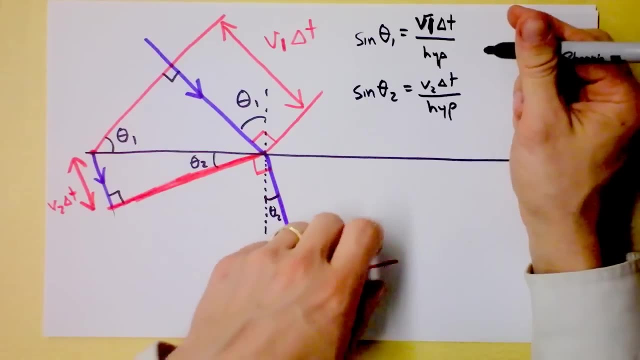 v one, The speed on side one times delta t, and this side's going to be the speed of side two times delta t, and I have to divide it by the hypotenuse. Now check this out, I could solve this for hypotenuse or I could solve it for one over. 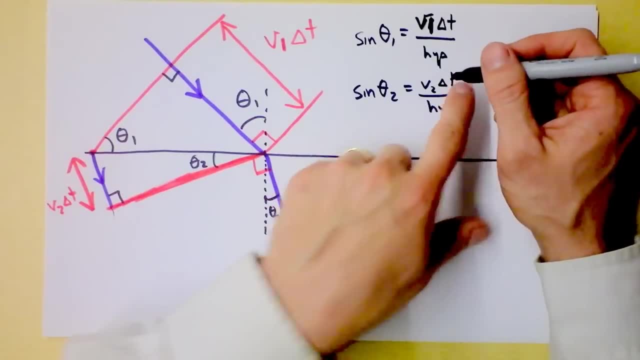 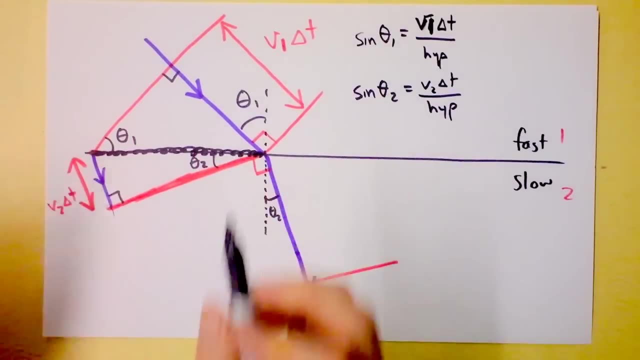 hypotenuse. I think that's what I'm going to do. You know that one over hypotenuse has to be one over hypotenuse because, look, this is the hypotenuse of both of them. It's the same length, so I can make the conclusion. check it out. I'm going to say that one over 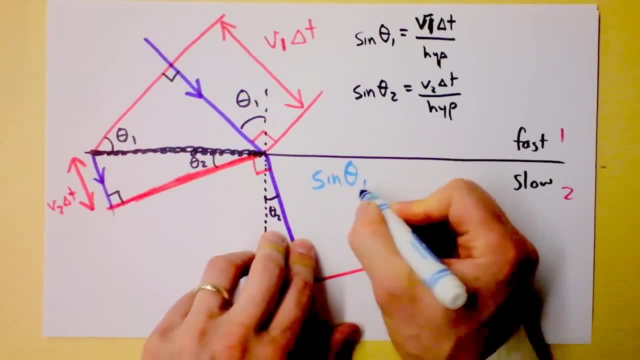 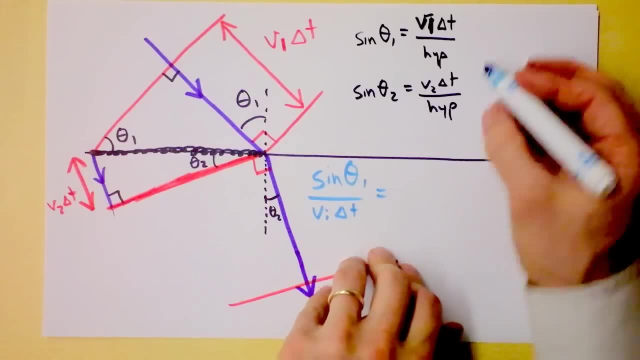 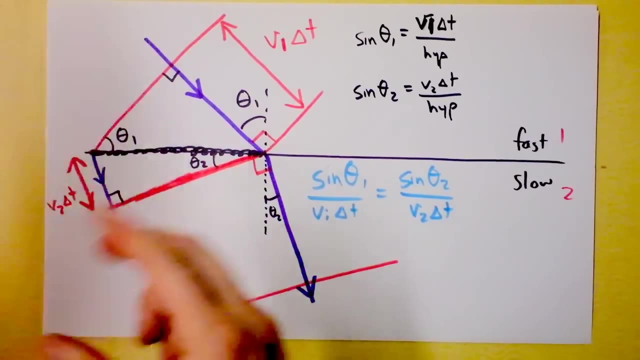 hypotenuse on the top equation says: sine of theta, one divided by vi, delta t is equal to the one over hypotenuse on the other side, which is sine of theta two divided by v, two times delta t, and we can immediately cross out the delta t's who needed them anyway. 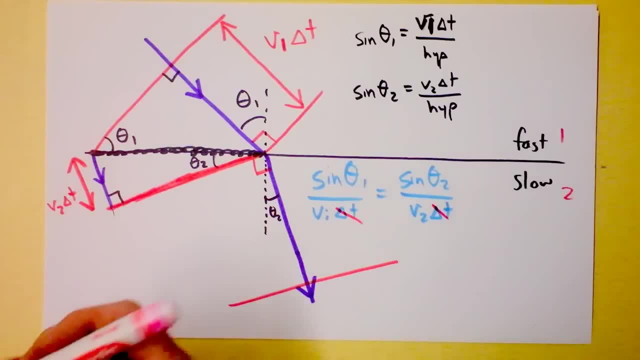 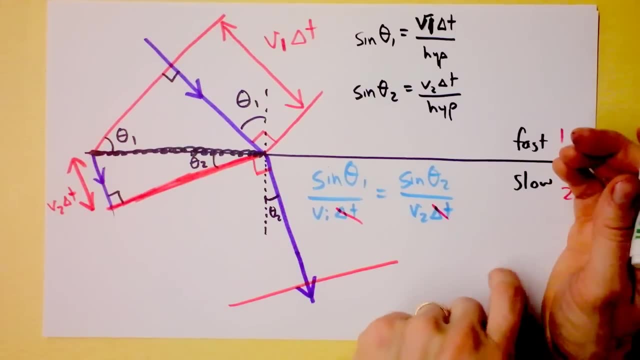 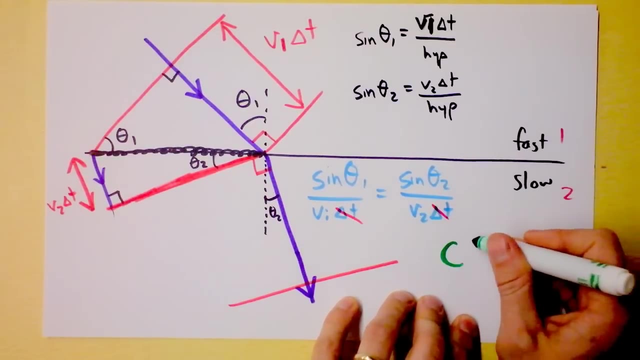 And then, well, I have to do something cool. right now, I'm going to define something called an index of refraction, And it tells me How refractive this area is right here. so here we go, I define index of refraction. well, I could write it like this: the index of refraction is: wait a second. c is not index of refraction. 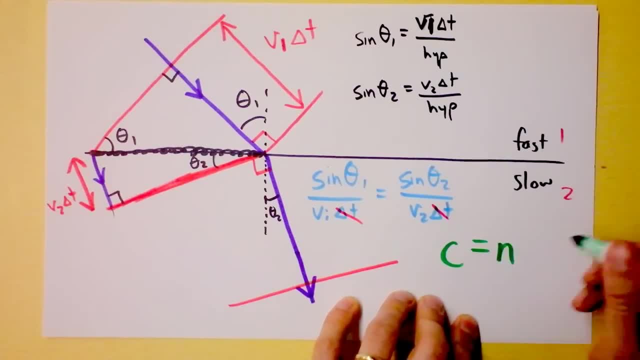 c is the speed of light. the speed of light is the index of refraction times the speed of light in the material. or, or I could say that the index of refraction is defined to be The speed of light divided by the speed of light in the material. now you know that the 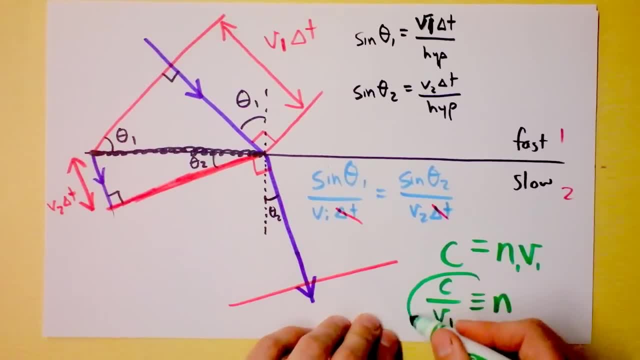 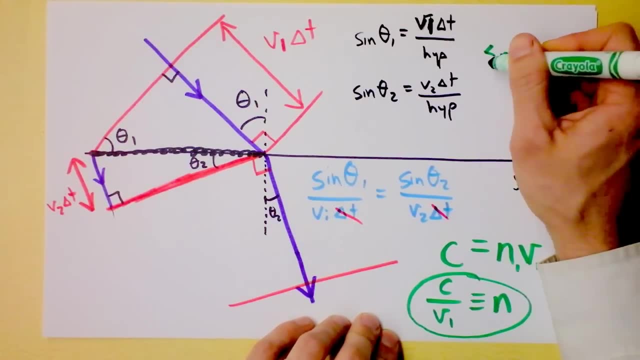 fastest light goes is when it doesn't have a material to go through, right. so you know that this index of refraction, what are we going to say? n is what's the smallest that n can possibly be. it's going to be greater than or equal to one, and it could be all the. 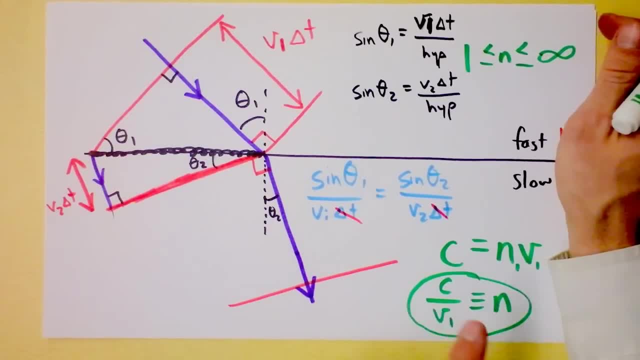 way up to infinity. yeah, I mean you can get objects that have infinity. whoa, if this is infinite, that means that light would stop in the material, and five, maybe ten years ago you couldn't have a material that did that. but I'm thinking about those Einstein condensates. 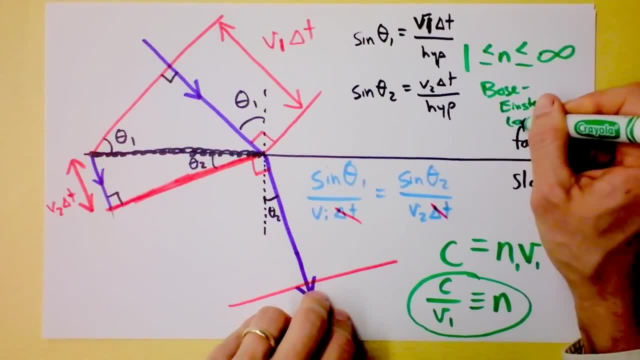 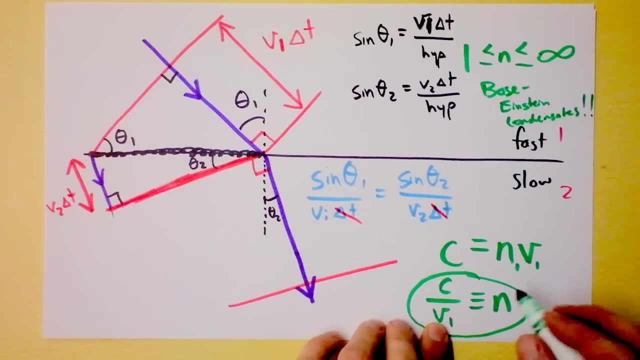 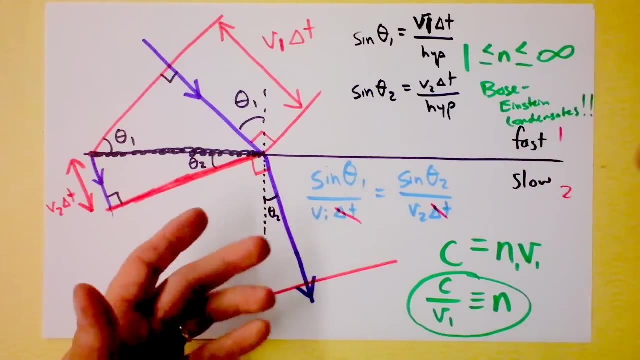 right now. you know that I am, And those suckers stop light. wow, if lights has a velocity of zero in that material, then the index of refraction material is in fact infinite. and it's very easy to make an index of refraction material of one or very close to it. if you just go through a vacuum, then 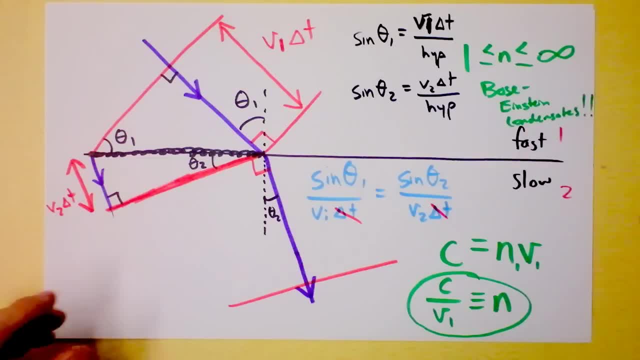 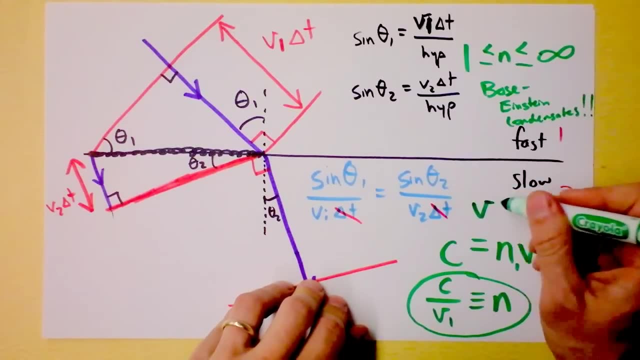 light will be going at light speed in a vacuum by definition. and so that you're cool now I'm going to plug this into right here. If I rearrange Equation one final time and I say: the velocity of light is equal to the speed of light divided, 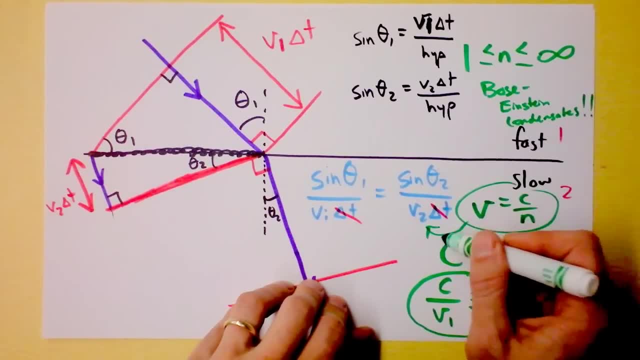 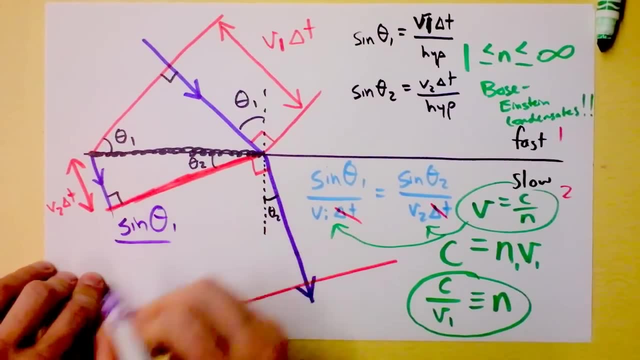 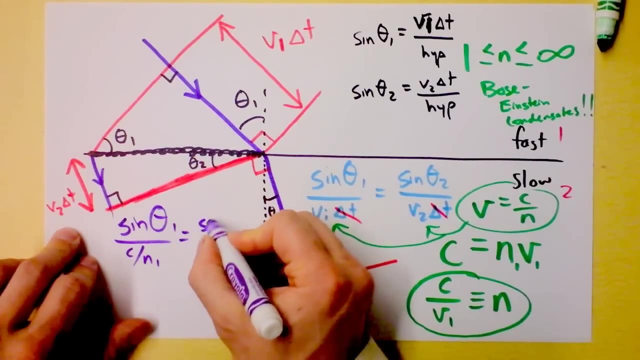 by the index of refraction. I could then plug it into this equation and this equation and I hope to find something that might be useful. I find that sine of theta one divided by- wait for it, this has got to be C over n one- equals sine of theta two divided by C over n two. 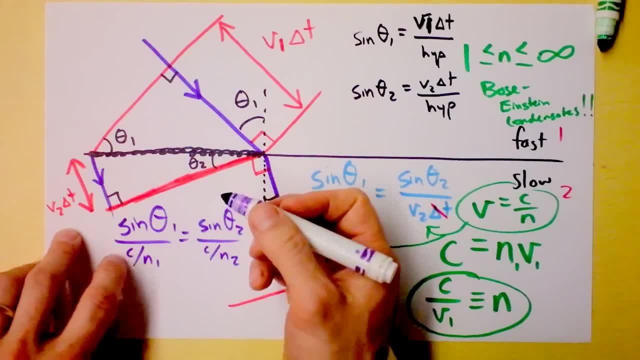 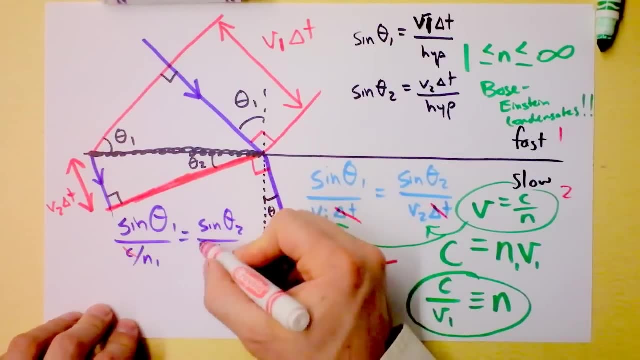 because that's what. v two is C over n two: the speed of light in a vacuum is the speed of light in a vacuum. so if I simplify all of this, I get my C's cancelled out. see, there's a C here and there's a C there. 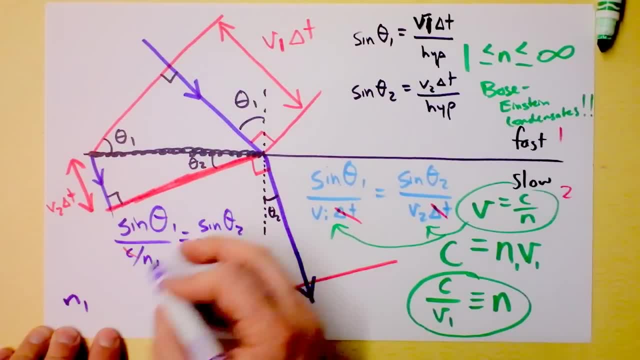 and I get n one. now this is in the denominator of the denominator, so it's n one times sine of theta one, is n two times sine of theta two. this is how- whoa sorry about that dot there. This is how you determine The angle.